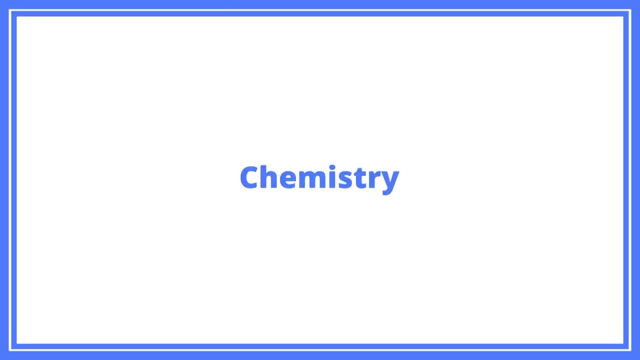 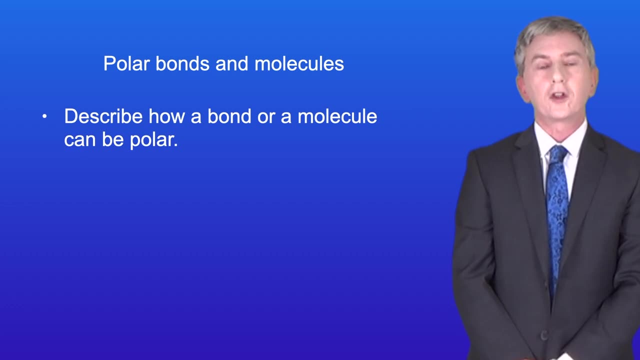 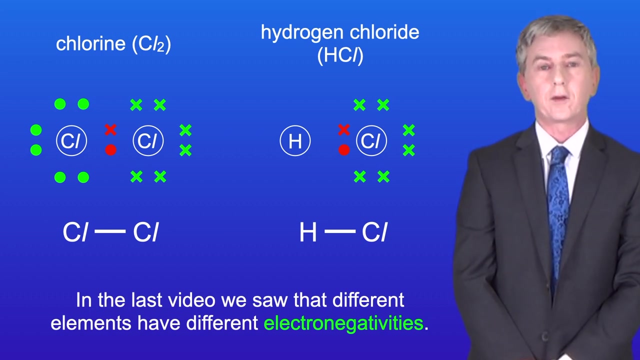 Hi and welcome back to Free Science Lessons. By the end of this video you should be able to describe how a bond or a molecule can be polar. In the last video we saw that different elements have got different electronegativities. Electronegativity is the ability of an atom. 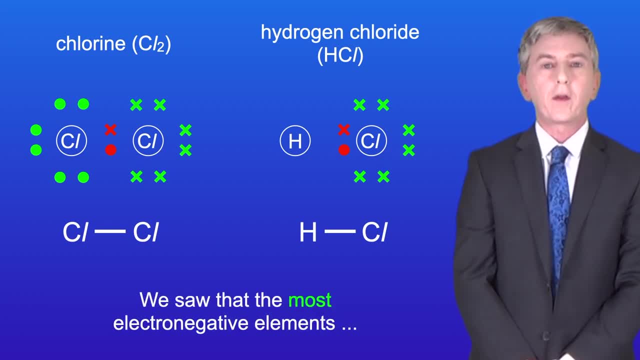 to attract the pair of electrons on a covalent bond. We saw that the most electronegative elements were at the top right of the periodic table. I'm showing you here the chlorine molecule, Cl2, and the hydrogen chloride molecule, HCl. Looking at the chlorine molecule, we can 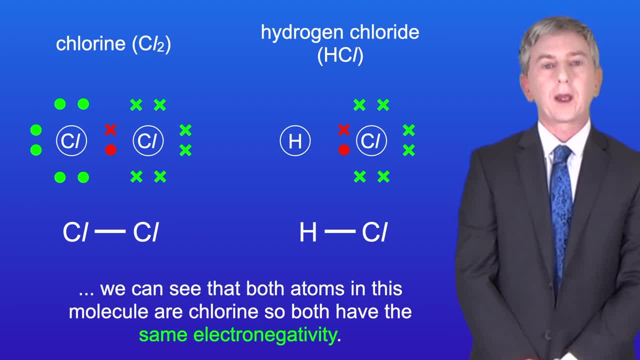 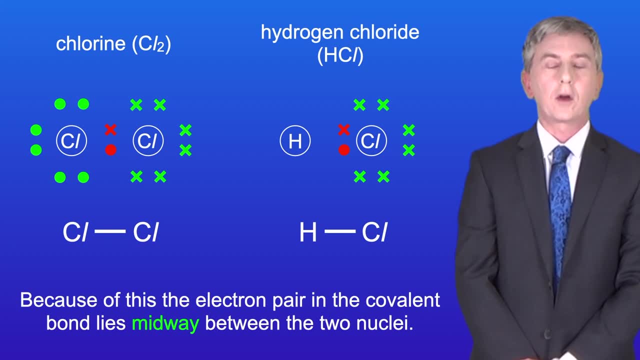 see that both atoms in this molecule are chlorine, so both have the same electronegativity. Because of this, the electron pair in the covalent bond lies midway between the two nuclei, and scientists call this a pure covalent bond. However, in the case of hydrogen chloride, 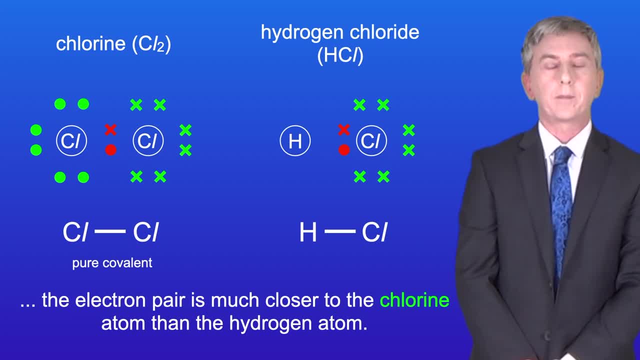 the electron pair is much closer to the chlorine atom than the hydrogen atom, and that's because chlorine has a greater electronegativity than hydrogen. Scientists call the separation of charge a dipole, and the covalent bond in hydrogen chloride is described as a polar. 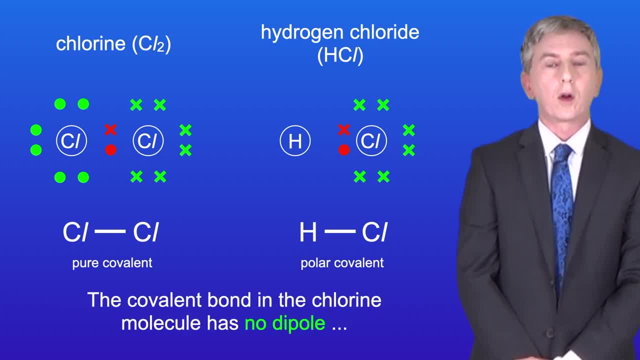 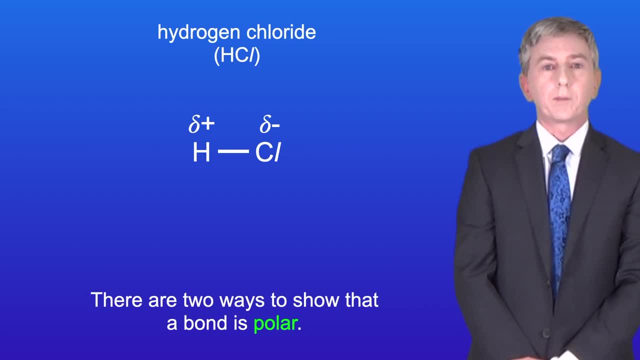 covalent bond. The covalent bond in the chlorine molecule has no dipole, so this is an example of a pure covalent bond. Now there are two ways to show that a bond is polar. The first way is to write delta positive and delta negative to show the charges. Delta means that the 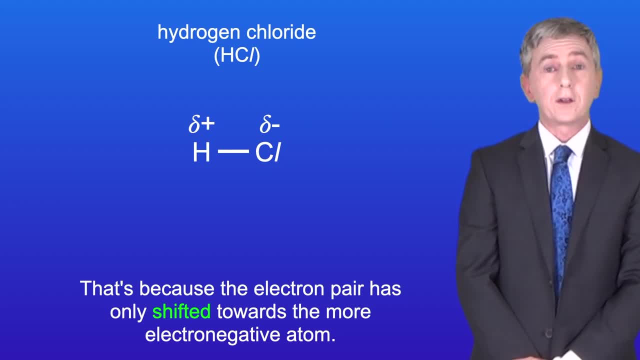 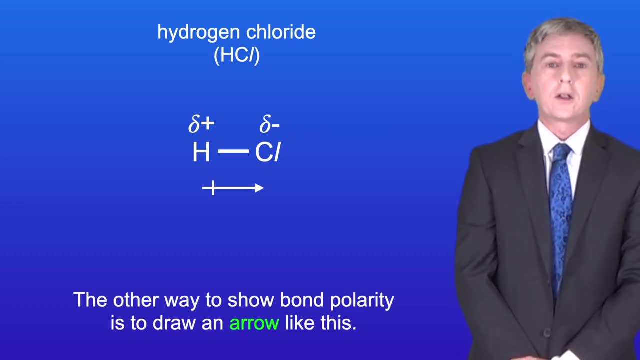 charge is small and that's because the electron pair is not polar and the charge point is has only shifted towards the more electronegative atom. The delta negative sign will go on the more electronegative element. The other way to show bond polarity is to draw an arrow like this: 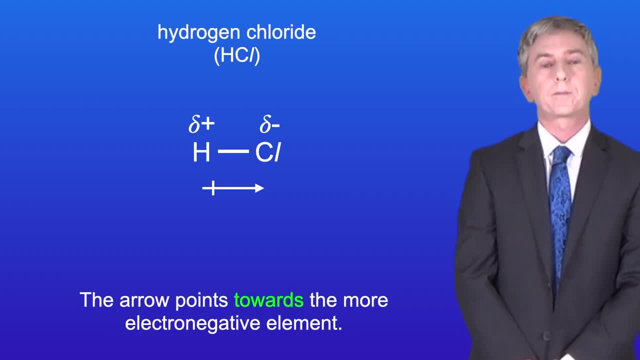 and the arrow points towards the more electronegative element. Now, because hydrogen chloride only has one bond and that bond is polar. this means that the hydrogen chloride molecule has an overall polarity. Scientists call this overall polarity the dipole moment. But what about molecules with more than one bond? 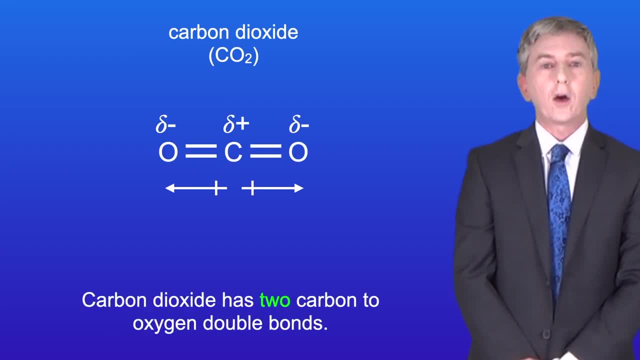 I'm showing you here the molecule carbon dioxide. Carbon dioxide has two carbon to oxygen double bonds, and both of these bonds are polar. However, these bonds point in opposite directions in a straight line, so that means that the dipoles cancel each other out.